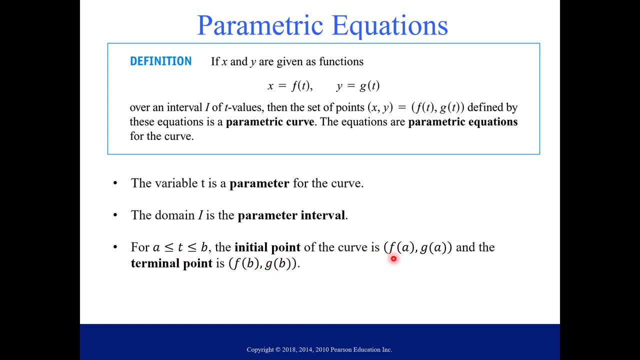 calling it Pelc como, and he'll say: oh, this is five exponents or times this. So what that first variable is called is called the parameter interval for t between a and b. so notice, this is a closed interval for your parameter. the initial point on your curve is when you plug in a for t. okay, into. 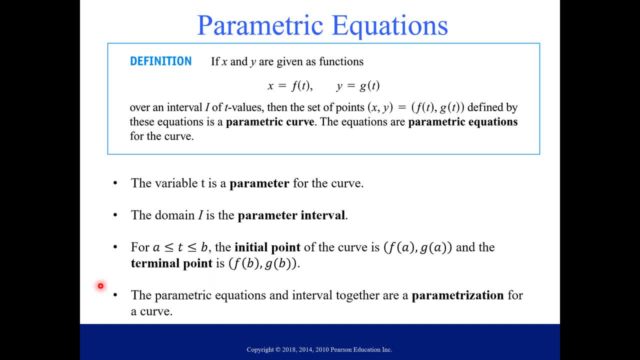 your functions for x and y and then the terminal point on your curve. so where your curve ends is when you plug in b for t into your functions worth x. a plus t, minusing that value of x is monde. And then parametric equations and the interval of the parabola. anybody who does any Suit orator? 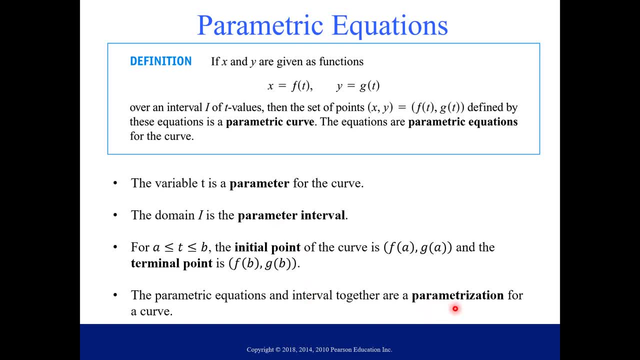 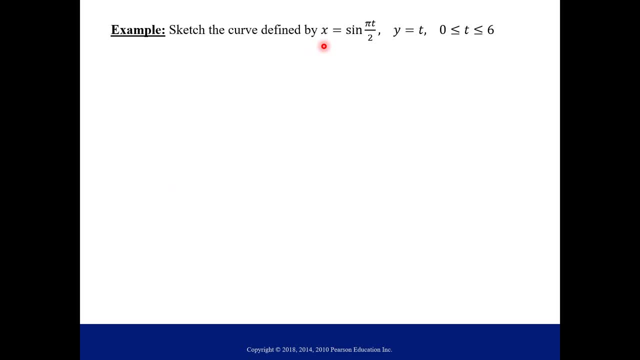 parameter interval together. That's what makes up the parameterization for a curve. So let's look at an example. Sketch the curve defined by x equals sine of pi times t over 2, and then y equals t, and this is for t between 0 and 6.. So this is an example right here given to you as 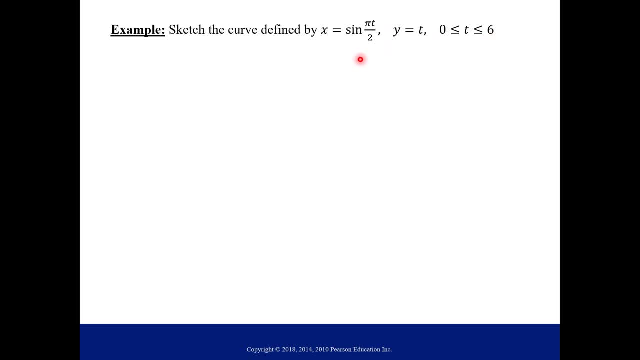 parametric equations. This is a parameterization. It has functions for x and y and then an interval for t. So let's see what this curve looks like. We're just going to start with our initial t value of 0, plug it into our function for x. we find out that x is 0. We do the same thing for y. plug in. 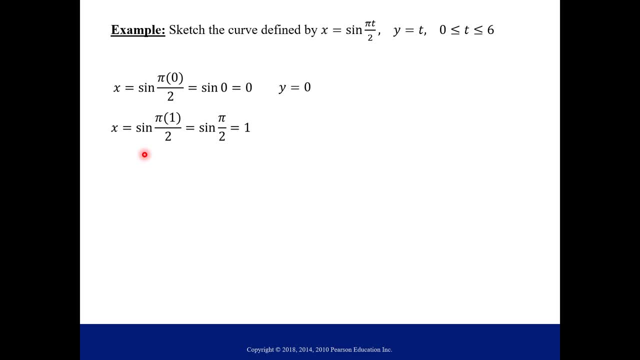 t is 0, and we get that y is 0. We'll do that again for another t value. So I'm just going by whole numbers. so I plug in 1 next. So sine of pi times 1 over 2 is just sine of pi over 2,. 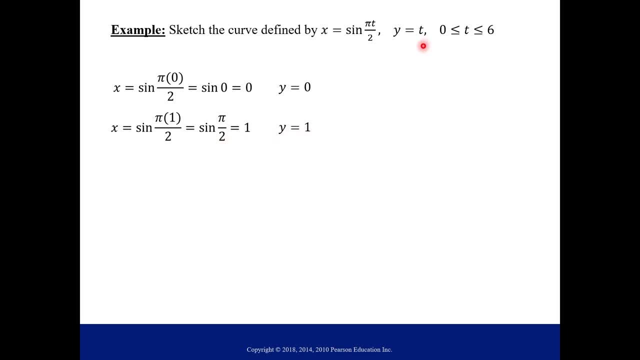 which is 1.. And then y is just t, which was 1 in this case. So if you do this for just the whole numbers, for your interval 0 to 6, you'll get the following x and y values. You can pick more numbers, You don't. 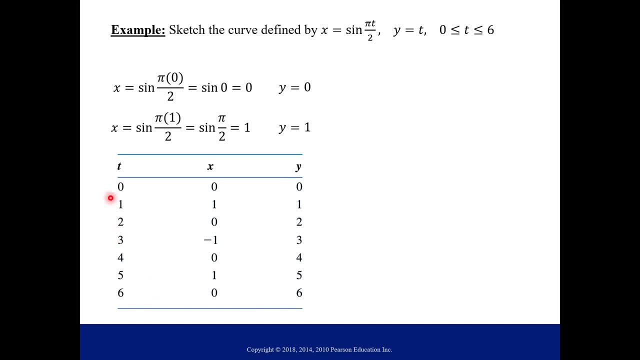 have to just stick to whole numbers, and I'll show you another example where we pick more. So take a look at this curve. So our particle, or the motion that this curve is describing, starts down here, at the point notice it's 0 comma 0. Then it moves to the point 1 comma 1, and then it keeps going as. 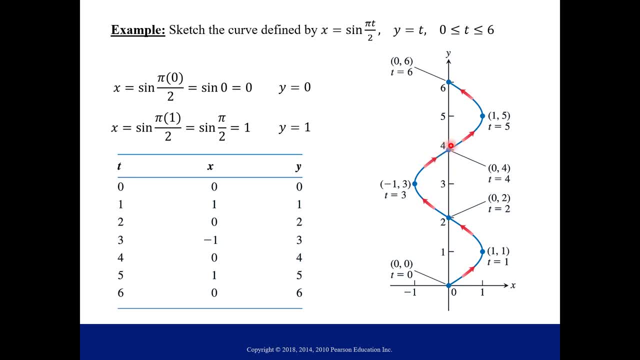 we plug in a different t value And as t is increasing the particle would be moving up this curve. So this is actually maybe not enough t values for you to know that this curve would have this kind of bendiness to it. So you might need to plug in more in the future if you have. an uncertainty about how much you want to plug in, So we're going to plug in more in the future. So this is actually maybe not enough t values for you to know that this curve would have this kind of bendiness to it, So you might need to plug in more in the future if you have an uncertainty about. 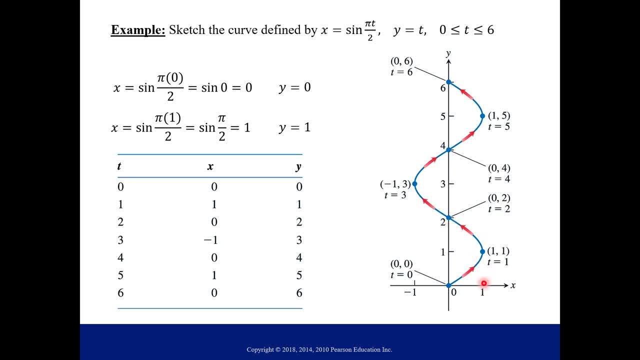 how to draw the actual curvature of this curve. So this is our first example. Notice it is on a closed interval for t. so we start at 0, that's our initial point and we stop up here at 0, comma 6,. 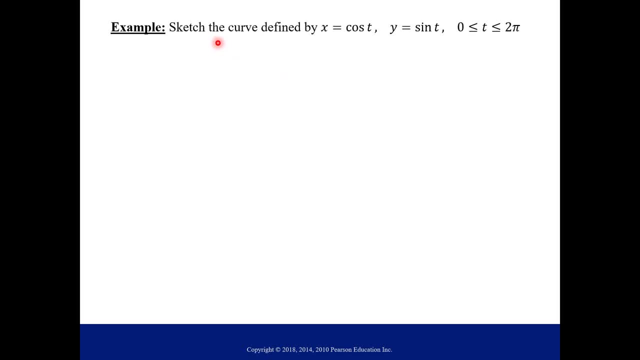 and that's our terminal point. Let's try this one here. We're going to sketch the curve defined by: x equals cosine t, y equals sine t, and this is for t between 0 and 2 pi. So we're going to start. 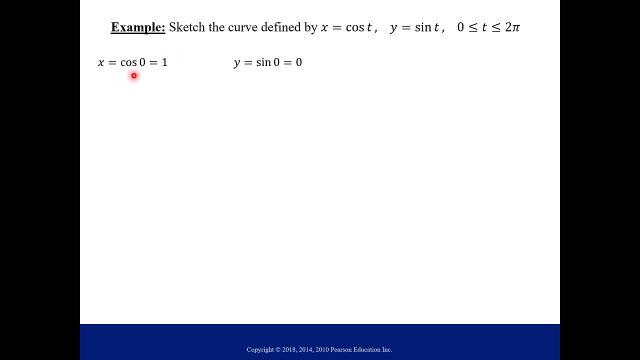 by picking t values. I'm going to just start with the very first one, which is: t equals 0. So I plug in 0 into my function for x, so cosine of 0 is 1.. I plug in 0 for my y function. 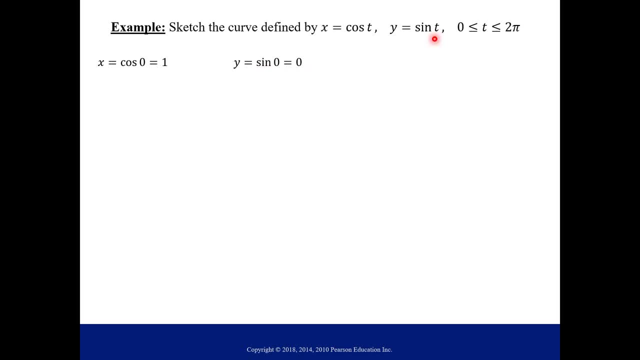 which is sine of 0, which is 0. And then I keep doing this. You can pick any numbers for t and you pick them in increasing order, and the next one I chose is pi over 4.. So cosine of pi over 4 is about 0.71, and that's going to be our x coordinate, And then sine of. 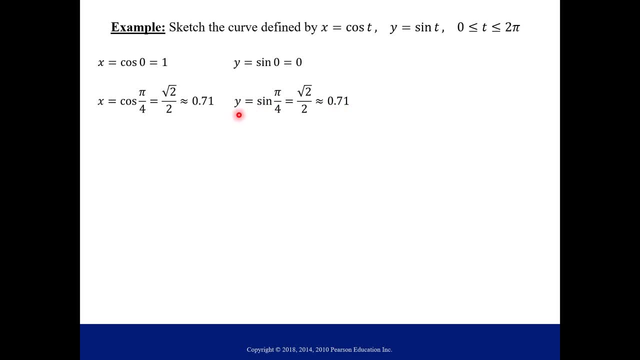 pi over 4 is about 0.71, and that's our y coordinate. So we're going to have a point on our curve that this defines as 0.71, comma 0.71.. And then you pick another t value. The next one I picked was pi over 2.. I got my x value is 0,. 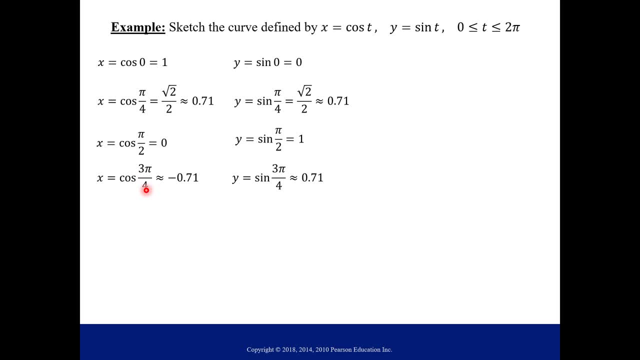 y value is 1, and then you keep doing that. Okay, let's do another one. I picked 3 pi over 4 for my next t value, and so we have negative 0.71 for x and then positive 0.71 for y. 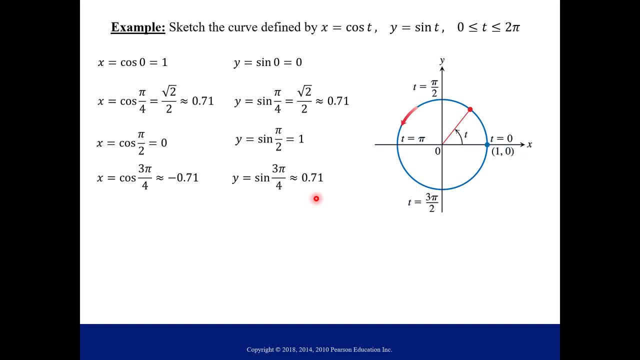 And hopefully this was kind of looking familiar as far as my values were concerned, and you might recognize that we were actually moving along the unit circle here. So what this was saying is that if you this path described by this parameterization, is that you have a particle, 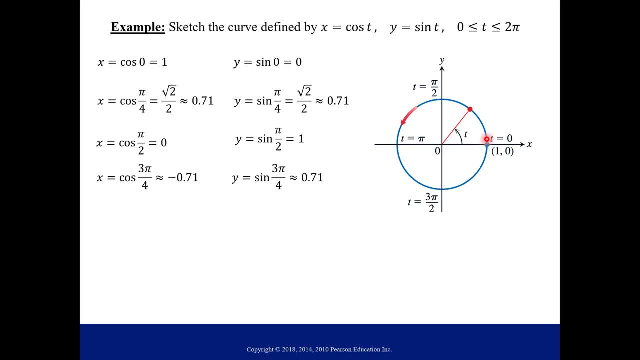 starting right here at 1 comma 0, and then it's moving along the circle. Okay, as t gets bigger, t increasing, you're actually moving counterclockwise Around a circle. And then, because we're told that we should stop with, t is equal to 2 pi. 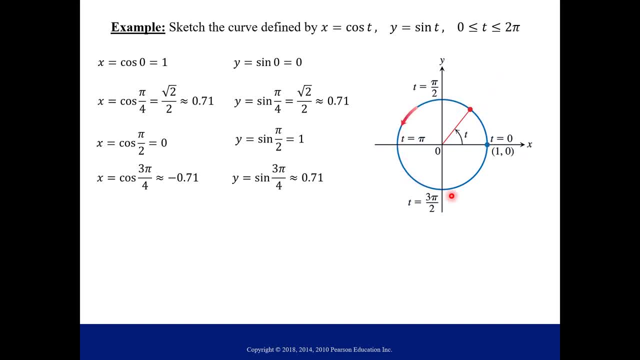 it's one tracing of this circle going counterclockwise. Now, this is, like I said, the unit circle. Okay, so just the other way to describe this- would be the way you're most familiar with it most likely- is: x squared plus y squared equals 1.. 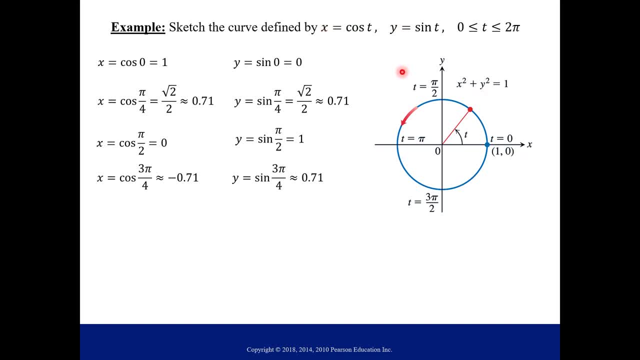 But this is the parametric way of describing this circle. So in general, the parameterization where x equals a number times cosine t, I'm calling that number a and then y equals the same number times sine t. This actually just describes a circle, but a counterclockwise motion along. 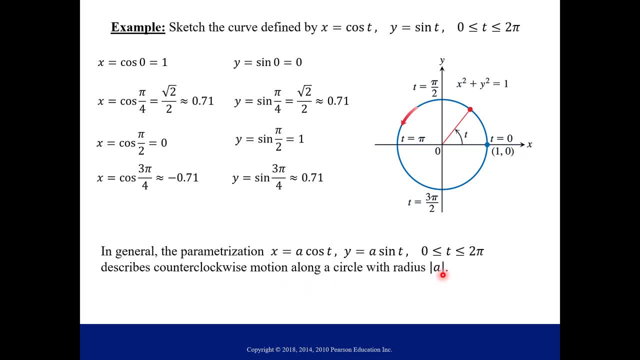 that circle where the radius is a. So in this case this was radius 1.. If there was a number like 5 in front of cosine and sine, that would have been a circle with radius 5.. So in general, this is the parameterization of a circle. Let's try this example. We are going to find a parameterization this time. 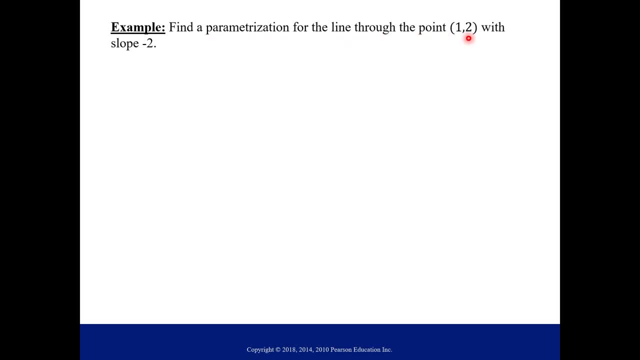 Parameterization, this time for a line through the point 1, comma 2, with slope negative 2. So this is new, because I've been giving you the parameterizations. this time We're finding it, So let's start with what we know about lines. This is our. 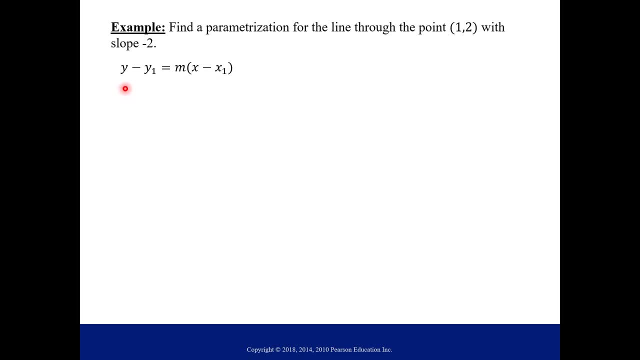 Point slope form of a line. you maybe you remember this from algebra, And so let's plug in our values. We know that y is 2, X is 1, and then our slope is negative 2, So what you're gonna do here is you're gonna pick. 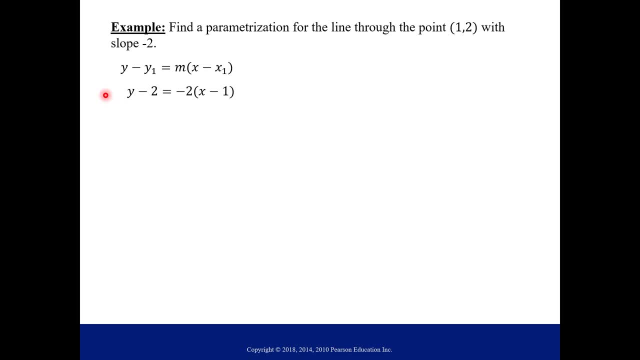 Some possibility for T and I'll show you that there's more than 1, so we are going to let T Equal X minus 1. I'm choosing this quantity in the parentheses. So if we solve for X, because remember what we're looking for in terms of a parameterization- we want X equals something. 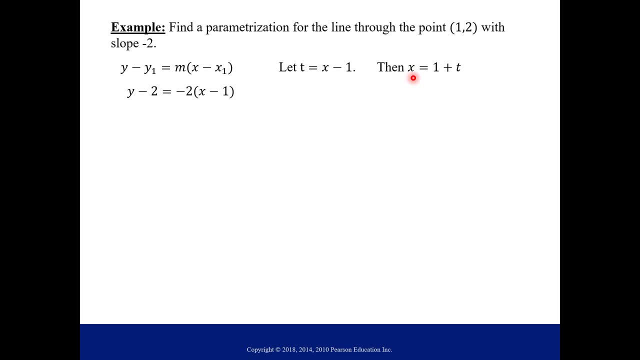 Y equals something in terms of T. So we solve for X, we get: X is 1 plus T, and then we move on to figure out what Y is. So we know this equation that we just had written down, And then we just decided that in the parentheses, X minus 1 is what we're calling T. 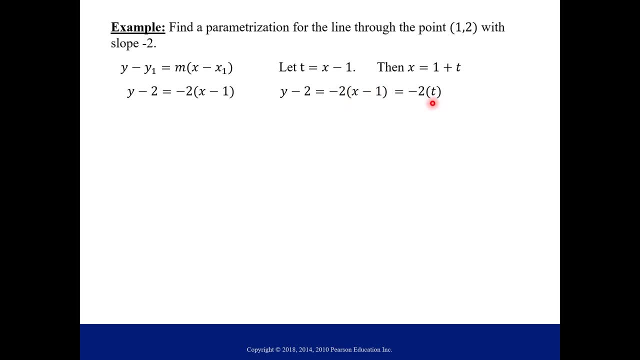 so you just replace the parentheses X minus 1 with T, and So you have that Y minus 2 equals negative 2 times T, And then, if you solve for Y, we get Y equals 2 minus 2 T. So then a parameterization for the line. 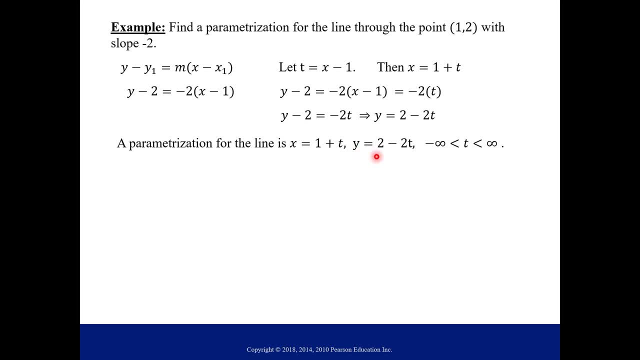 Is X equals 1 plus T. Comma Y equals 2 minus 2 T, and then this is a line with no kind of closed interval that we're told about. So this is for T, from negative infinity to infinity. This is a line that's going to continue on. 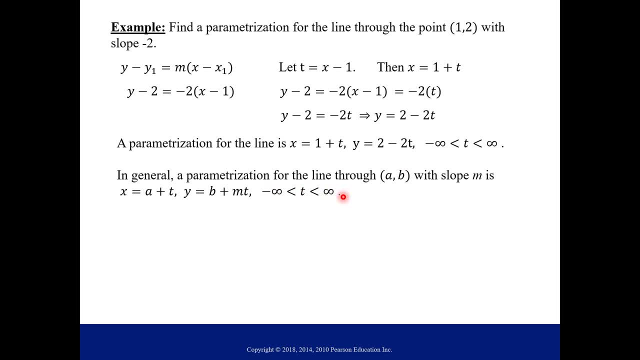 Now, in general, if you're asked to find the parameterization for a line through some point a comma B And you know the slope is M, Then in general you can use this setup where X is just the X value a plus T and then Y Is the Y value B plus your slope times T. so you can use this one in the future in general, 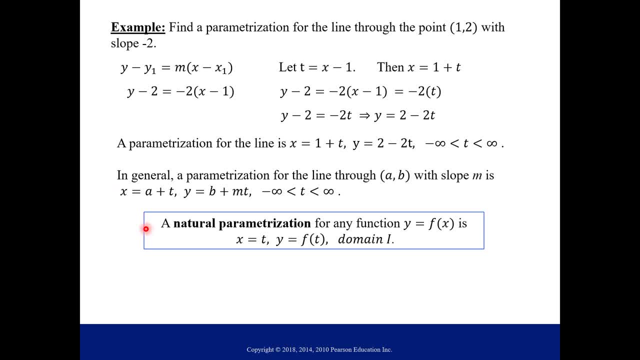 Now there is what's called a natural parameterization. for any function, F of X equals, Y is the function, and you can just say that X is T and then Y is just F of T, and That's not going to be on, whatever the original domain is for that function. So, using the example we just went over, take a look a. 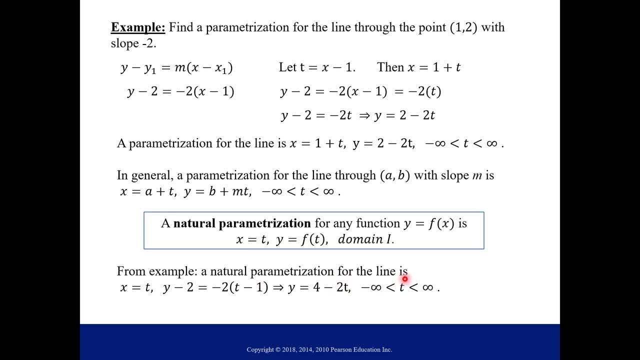 natural Parameterization for the line we just worked on is just to say that X is T this time. Notice it's different from what we initially chose. We chose: T is X minus 1.. So now X is T. So then you would just say from your equation back up here: Y minus 2 equals negative 2 times. 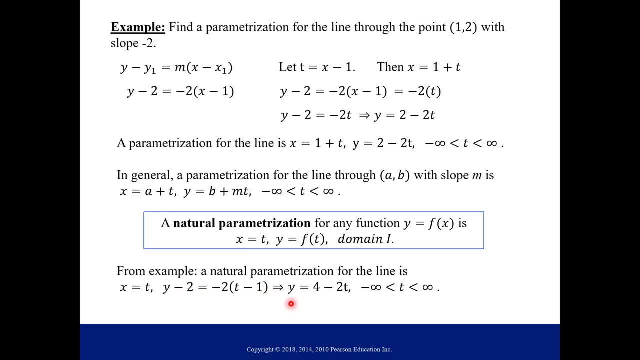 T minus 1, and then you just solve this for Y. So Y equals 4 minus 2 T. So this is a different parameterization For the same line. so I do want you to be aware that there are multiple parameterizations for the same curve. 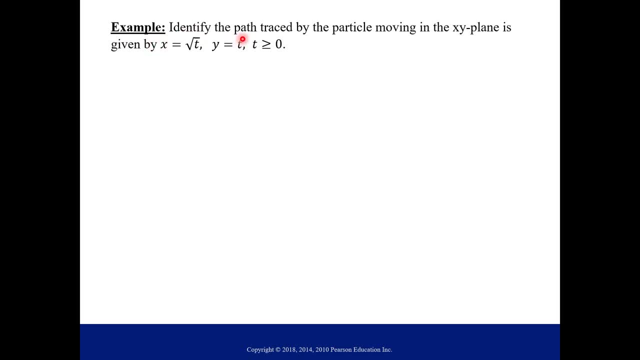 Let's do one more example. here We are going to identify the path traced by a particle moving in the xy plane. That is given by: X equals square root, T, Y equals T, and this is for T, That's zero or more. So what you're going to do this time is you're going to try to eliminate T.